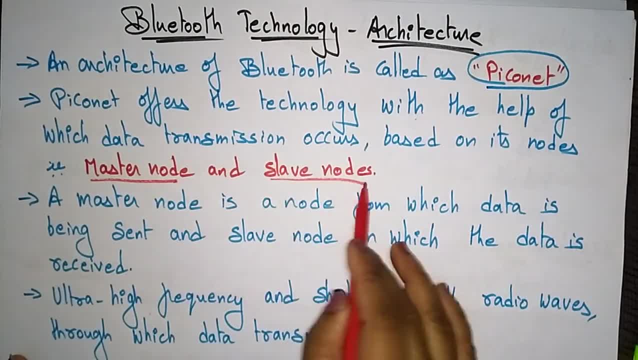 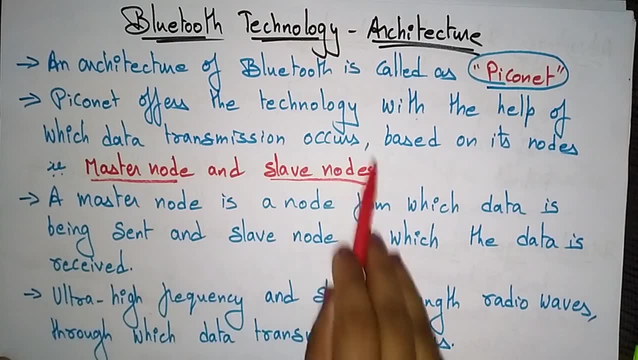 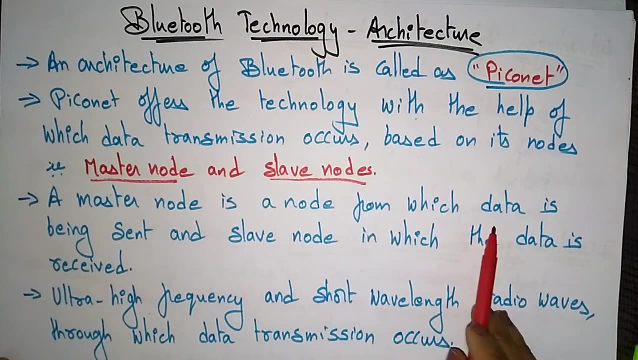 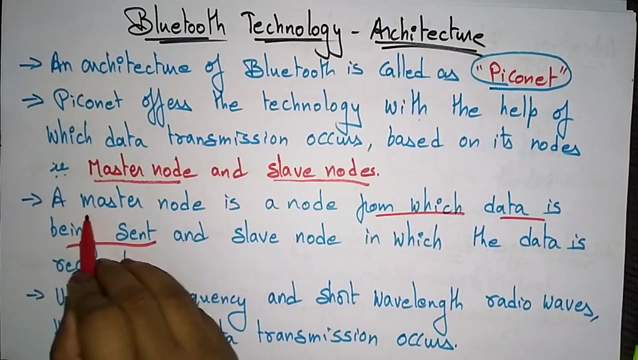 You call it as a master node and the receiving devices you call it as a slave node. So PicoNet offers a technology with the help of which data transmission occurs. Everything the data transmission will be based on this master and the slave nodes. A master node is a node from which data is being sent, So that I said from which data is being sent, as a master node, and the slave node is in which the data is received. The receiving node is a slave node. 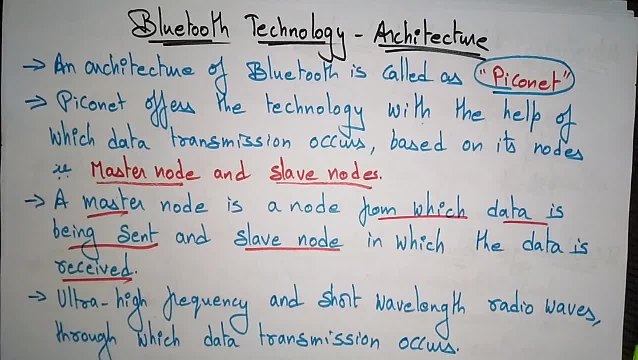 And sending node is a master. So here I am the master, I am sending the information to you and you are just listening what I am saying, that you are the slave. Okay. So here I am the master and so many slaves- or that means so many students- are there listening my lecture. Okay, So this arrangement completely is in the form of a PicoNet. So that is, the architecture of the Bluetooth is in a form of PicoNet. 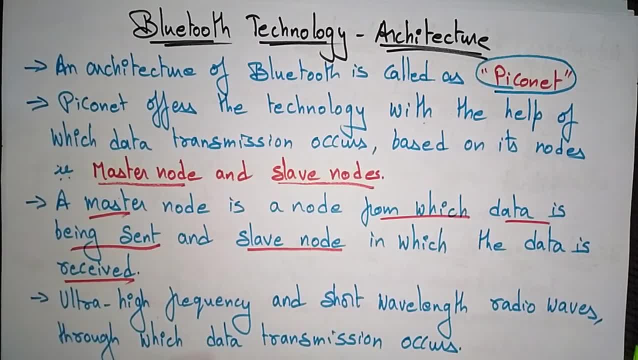 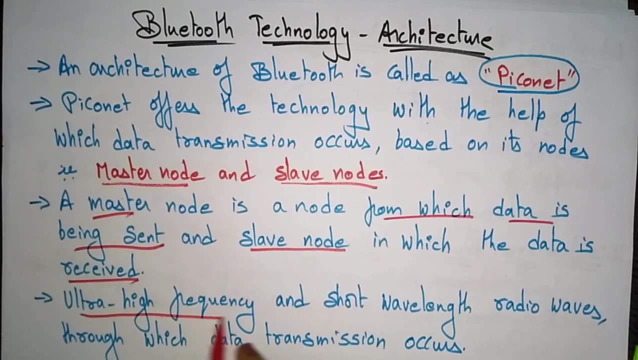 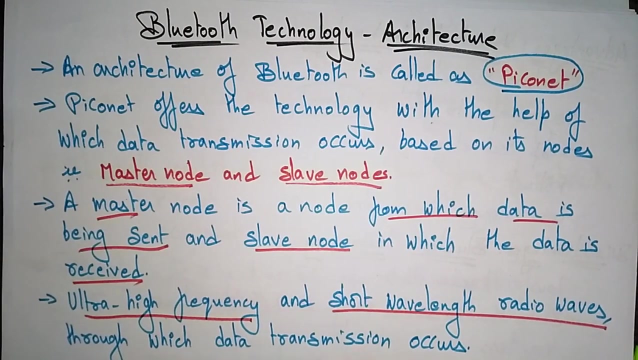 The ultra high frequency and the short Wavelength radio waves through which data transmission occurs. So you will get it out how the data is transmitting from one node to the different nodes. in the Bluetooth technology We are saying it is a wireless communication. So in the wireless how it is going to, a ultra high frequency will be there and the short wavelength radio waves. with the help of these two we are, the data transmission can be occurred. 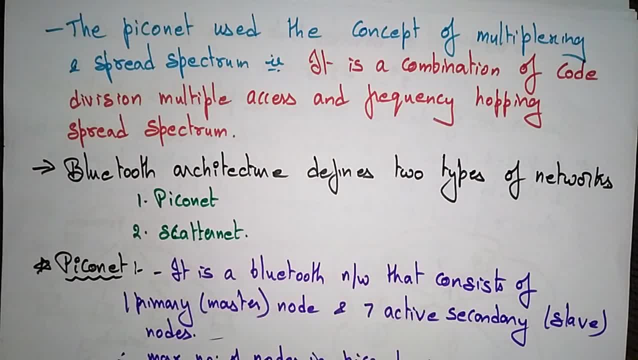 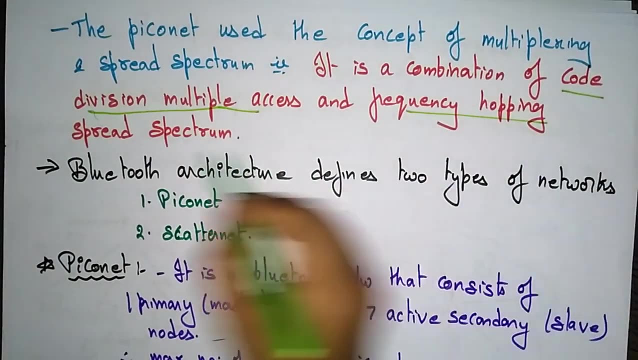 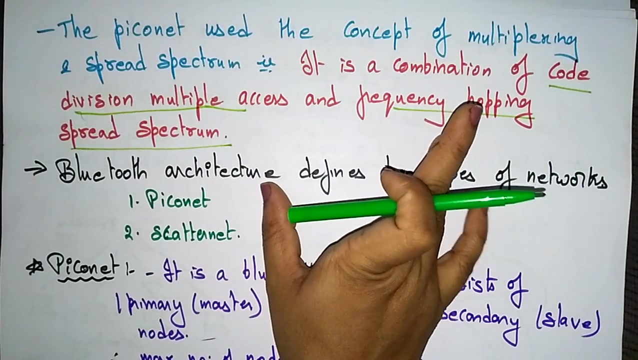 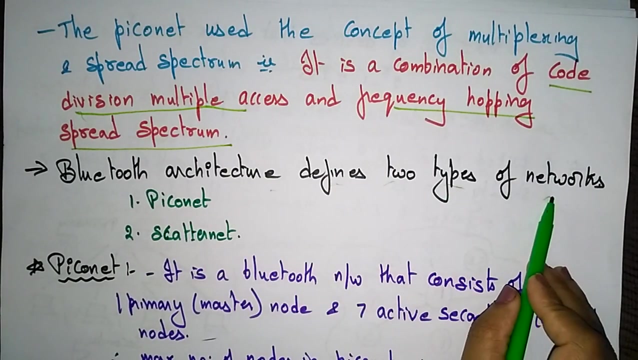 The PicoNet used in the concept of multiplexing and the spread spectrum, That is, it is a combination of core division, multiplex and frequency hopping. So here in the Bluetooth technology we are using the two concept. One is the core division- multiplexing access, and the frequency hopping- spread spectrum. So the complete structure, the master and slave structure, will be established based on this multiplexing and the spread spectrum technology. The Bluetooth architecture defines two types of networks. So before going to know about this, 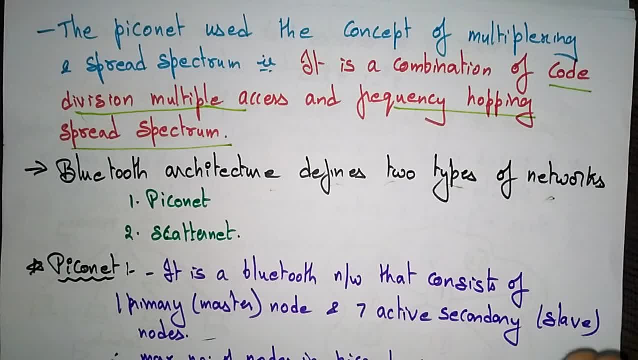 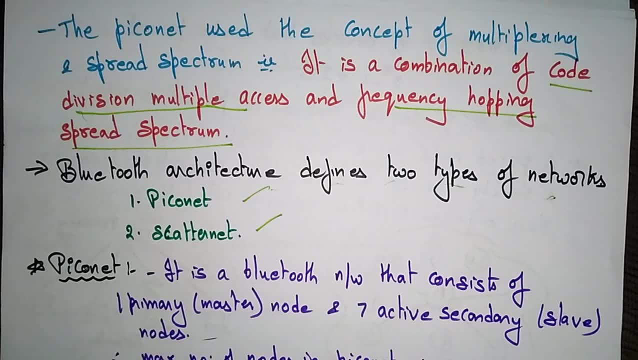 The, how the communication makes. the complete architecture is based on this two things: The PicoNet and the scatter net. So what does this PicoNet and the? what is a scatter net? Let's see it in clearly. I said a PicoNet is just a master and slave combination at. the sender is sending the information, The receiver is receiving the information. Let's see the PicoNet in clear. 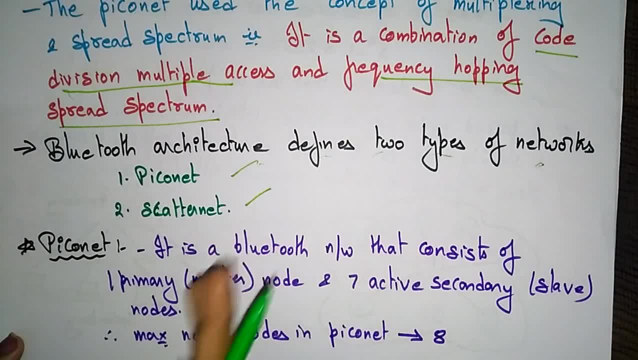 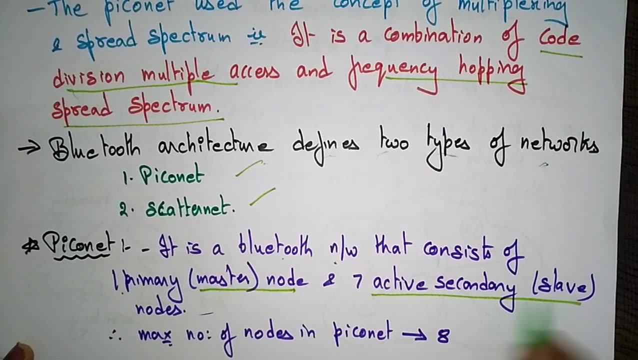 Because these are. this complete Bluetooth architecture defines these two types of networks. The arrangement of the network is in the form of either piconet or the scatter net. a piconet, it is a bluetooth network that consisting of one primary, only one master node is there and seven active secondary slaves are there. 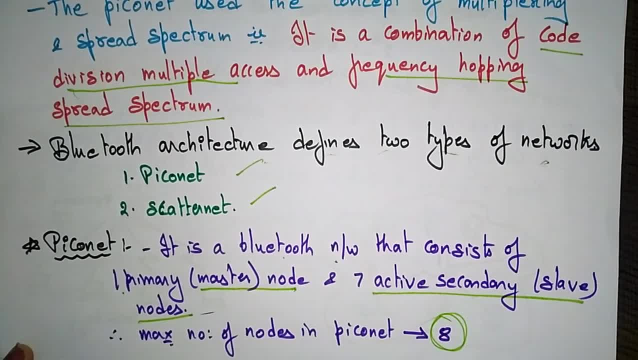 so maximum, the piconet consisting of only eight nodes. so i am the master, i am sending the information to you, so only the seven people at a time can use the information. the seven active secondaries will be there, that is, the seven active slaves are there because i want to be. 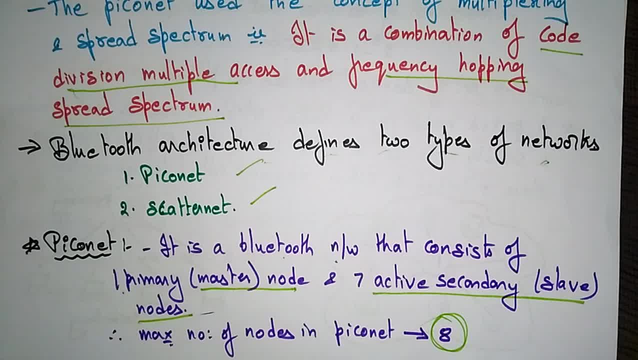 only communicate to only to the seven people. so i am just asking: okay, i can say, uh, give the lecture today only to the seven students. so those seven students are the slaves and i am the master and the remaining or just stationary. okay, so they are not in the network, so here only the. 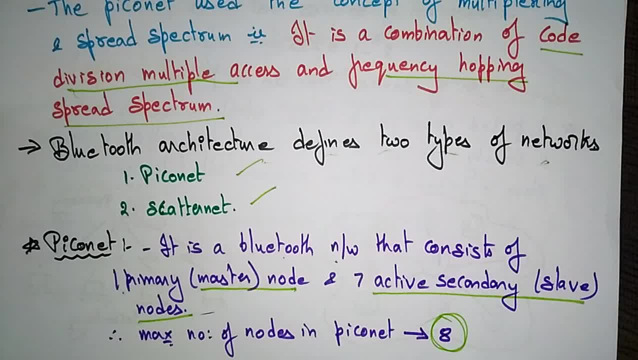 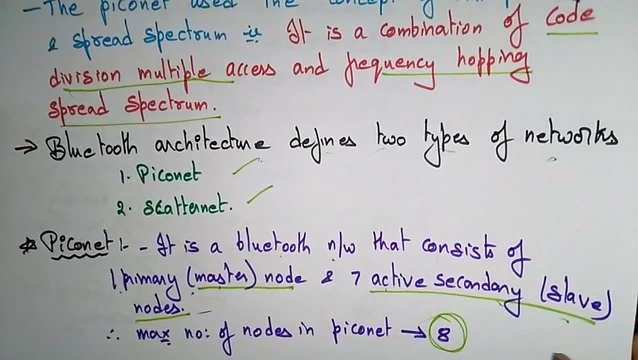 eight members are in the network: i myself and the other seven members. so Here, the one who is sending the information is a master and the 7 remaining are the slaves We call it as a secondary. So the maximum number of nodes in the PicoNet, that is, in the Bluetooth, only 8 nodes will be participated at a time. 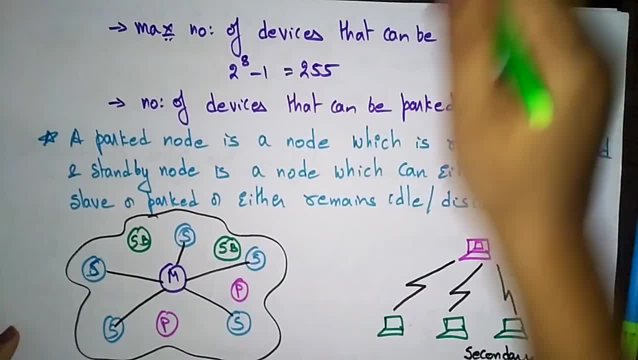 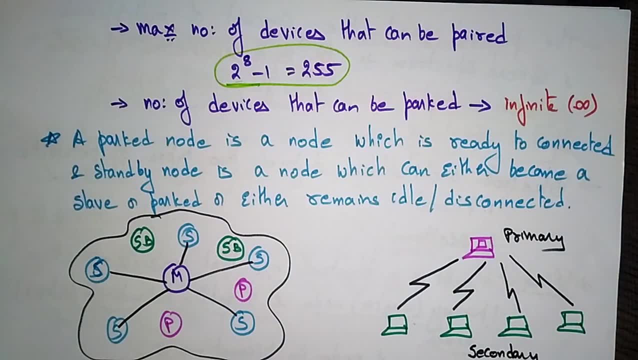 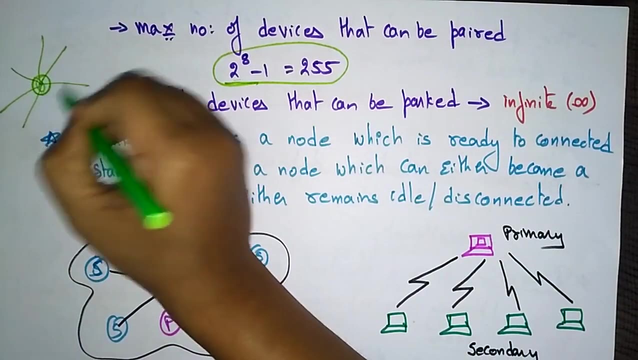 So the maximum number of devices that can be paired? So 2 power 8 minus 1, that is, 255 devices can be paired, Did you observe here? So only the 7 members can be. So here the master is there. Here, so many connections are there. 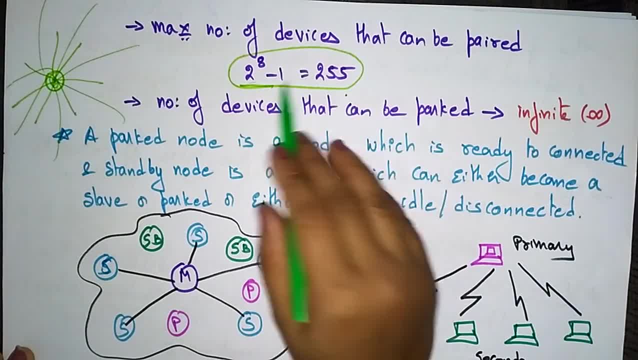 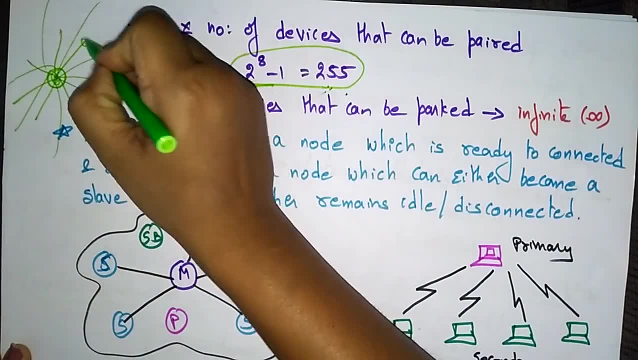 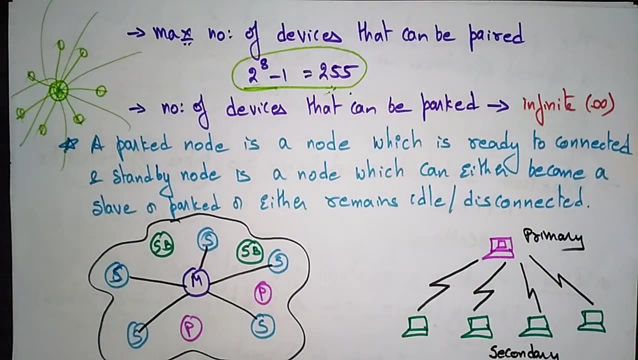 That is, 255 devices can be paired. Maximum number of devices that can be paired for a master is 255.. But I can only connect 7 members at a time. So after the completion of the Means, Whenever the our class is over the 7 members class. 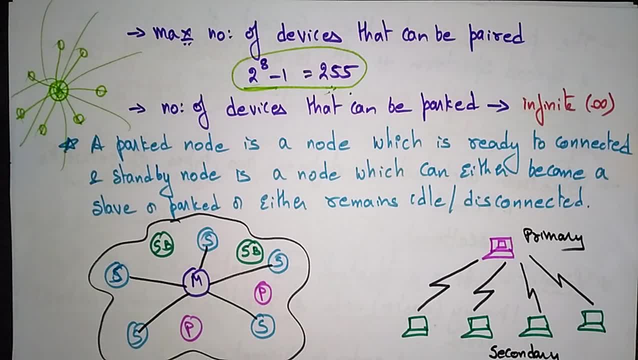 So these 7 members will be go out and another 7 members will be participated in the network. So they are still in the paired only. But even though they are paired, they are not in the network. So the maximum number of devices that can be paired is 2 power 8 minus 1, that is 255. 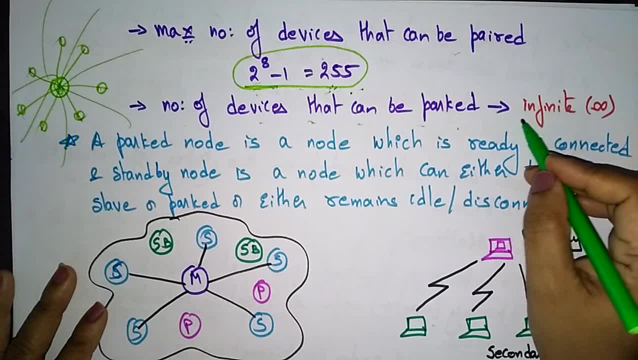 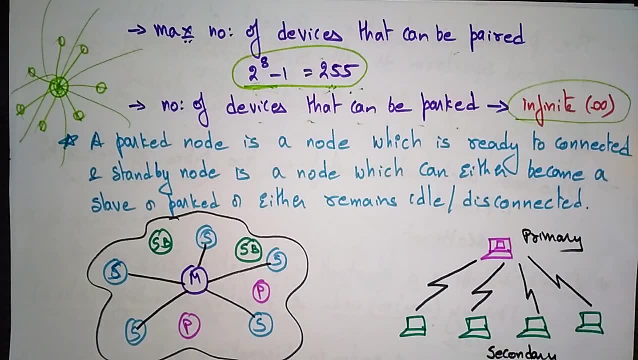 The number of devices that can be parked, That is infinite. Means the parked means waiting people. So many People can wait for me. means for listening the lecturer, So that may be infinity. You can't say the number, So that may be infinity. 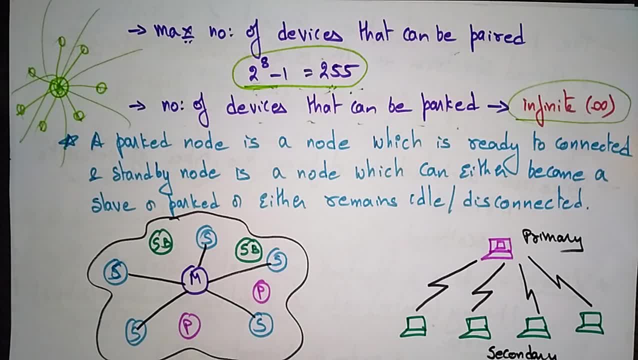 So whenever that 8 work is 7 work is over and the 7 will enter into the class and they will listen after that day. So whatever the student that is going out, another person will enter into that. So the maximum 8 nodes will be participating in the network in the Bluetooth technology that is a Pico net. 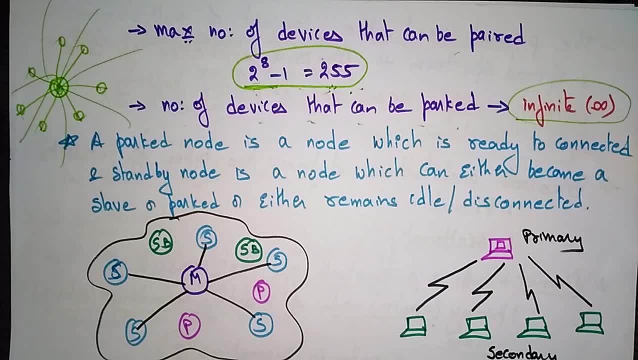 So here The infinite numbers should be there, but only the pair devices is 255, only The pair devices. you know the concept of the paired. whenever you are connected, that should be a pair devices. A paired is not a connected. whenever you try to connect it, then only it is participating in the network. 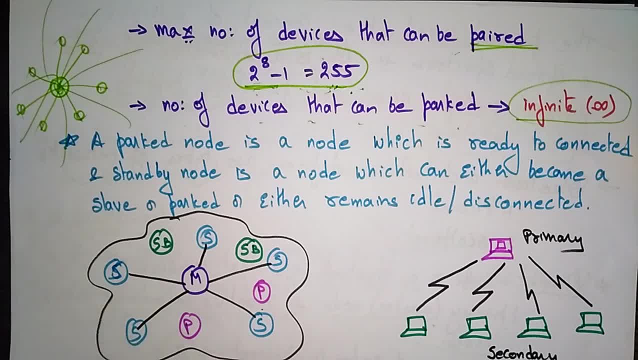 So I think you know the concept because whenever you switch on the Bluetooth the devices you are searching for the Bluetooth devices. So many devices will be paired Because you already communicated with them, So that will be paired one. So if you want to connect that devices, just click on that, then it automatically connected to that pair devices. 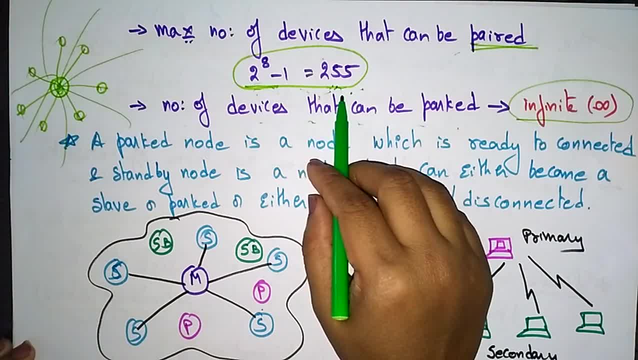 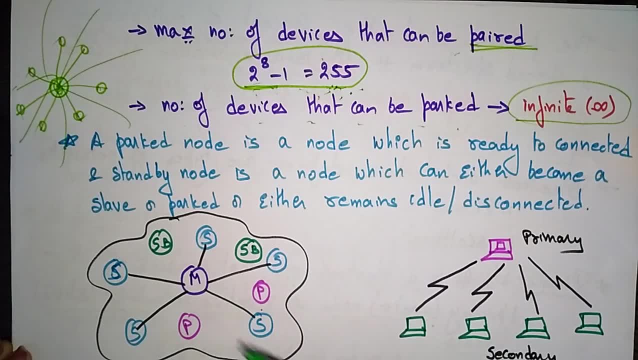 So the maximum number of pair devices in a Bluetooth is 255 and the number of devices that can be participated in the network that is, that is a Pico net, That is this: 8 total, 8 including master and the devices that can be parked- is infinite. 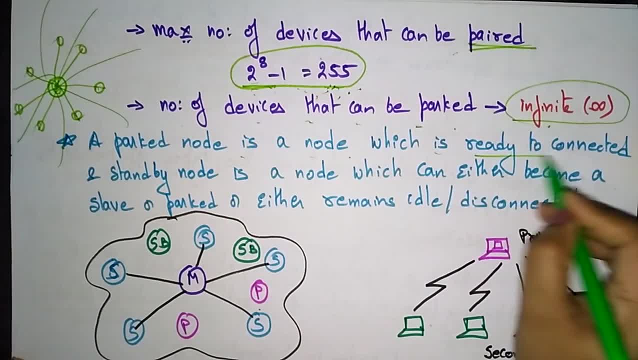 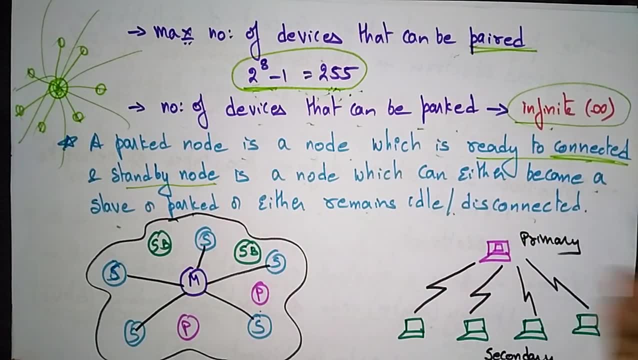 Okay, So the parkour node is a node which is ready to connect that. it is ready to connect it and stand by node is a node which can either become a slave or a park or either remain ideal or disconnected. So here two types of nodes will be there. 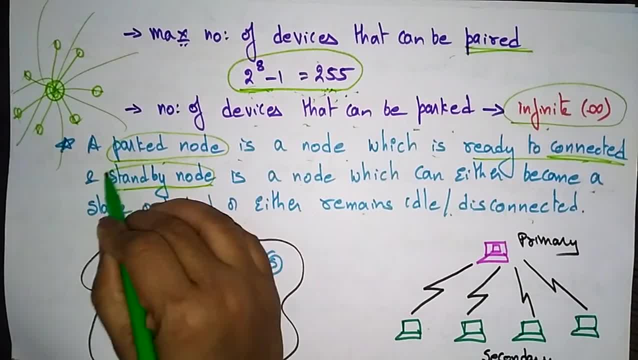 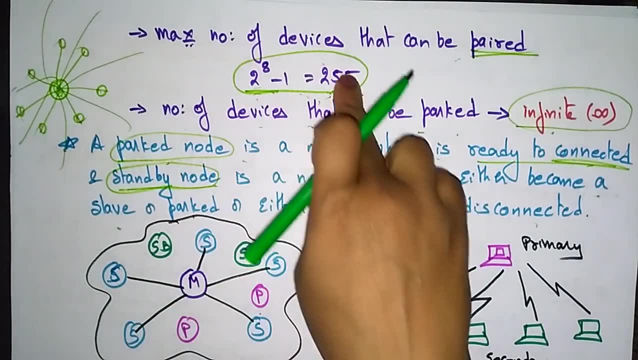 One is a parkour node and another is a standby node. Parkour node is ready to connect it. So whenever this 255 one is getting out, this parkour node can enter into this 255 pair devices. Afterwards it can enter into the network. 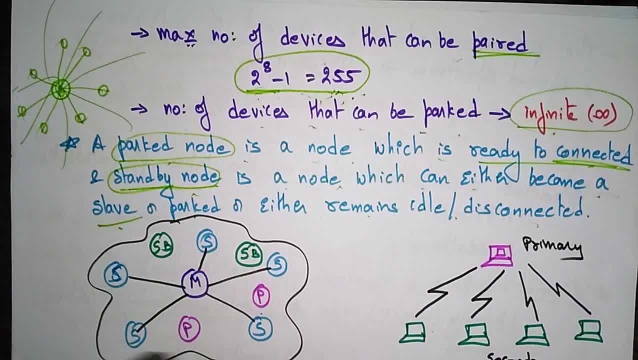 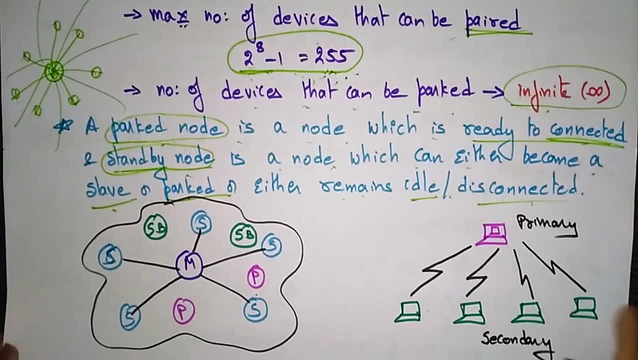 But standby node is a node which can either it become a slave in the future, or it can be a parkour, or it can be ideal or even disconnected. So let's see this Pico net structure. So here, this is the master, slave is there. 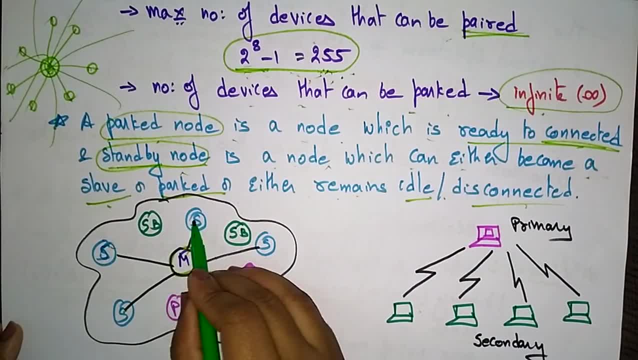 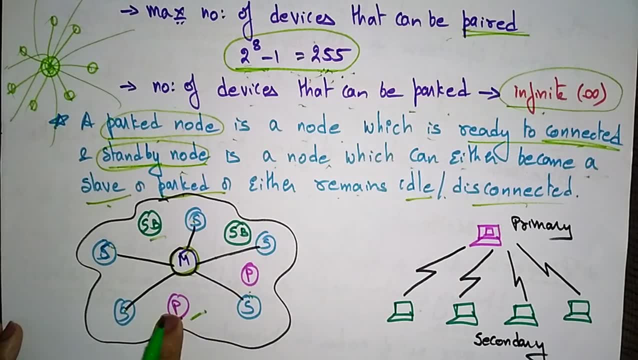 The master slave is connecting different slave devices on the network And here in this network, the standby nodes are there and the parkour nodes are there. So the standby nodes or parkour nodes are ready to connect it And the standby nodes may be connected. 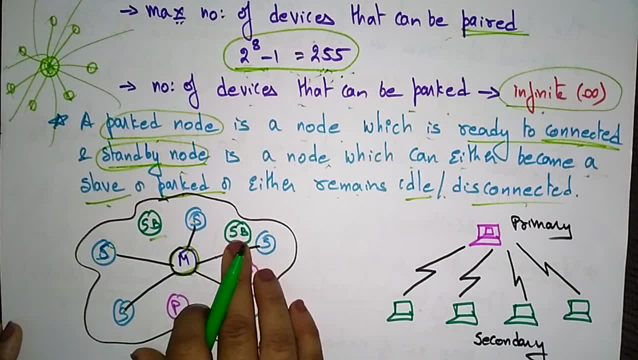 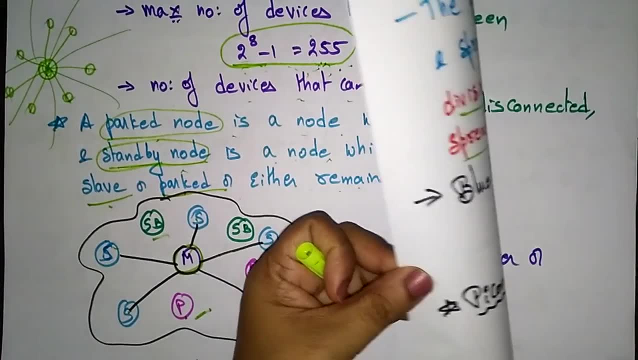 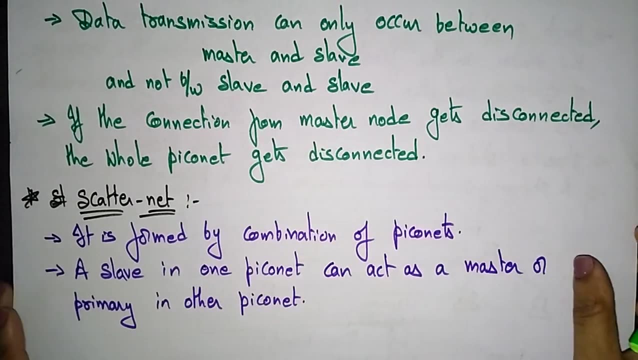 Or it may be a slave, or it may be a parkour, or it may be a disconnected node. So this is a primary and these are all the secondary devices. Okay, So this is about the Pico net And some more information I want to be shared with you. regarding a Pico net is: the data transmission can only occur between the master and slave. 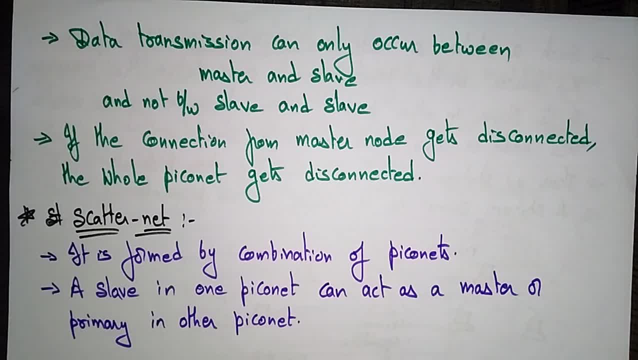 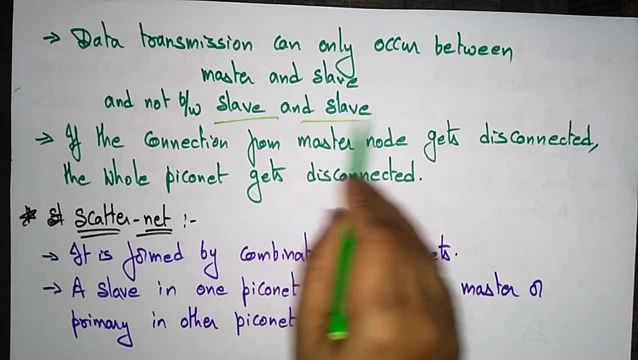 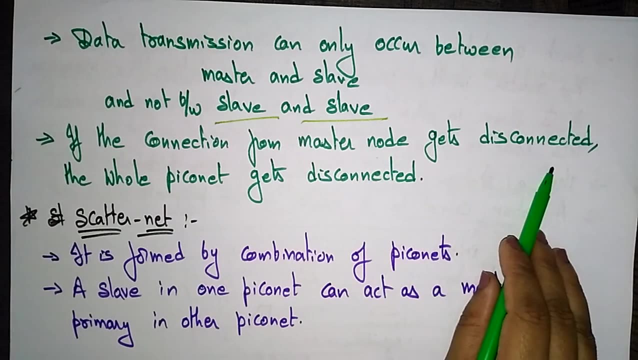 So only the master and slave data transmission will be occurred, not with the pair devices, only to the connected devices and not between slave and the slave. also you can't transfer the data between slaves only from master and the slave. communication will be there if the connection from master node gets disconnected. suppose i'm disconnected, i just 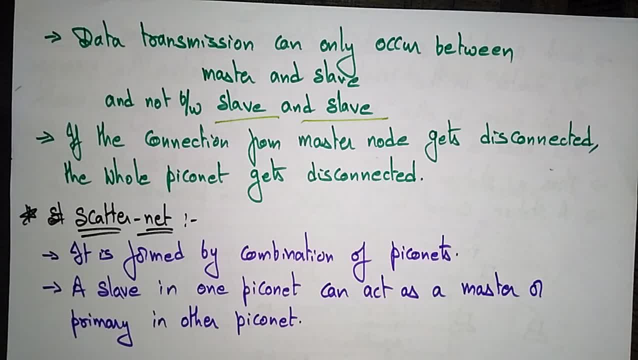 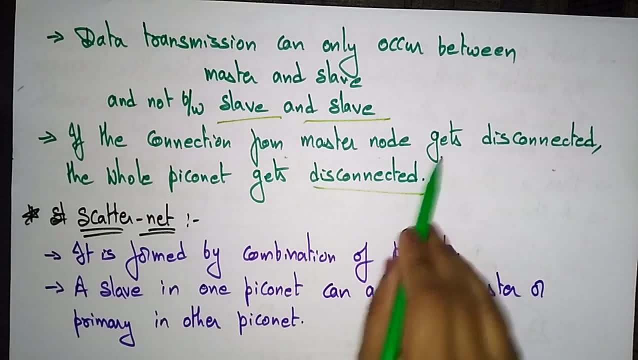 switch off my mobile. if suppose i stop my teaching, the whole piconets get disconnected. you're all disconnected, okay? so if the connection from master node gets disconnected, the whole piconets get disconnected whenever i'm taking the online classes. so if you're all reasoning, 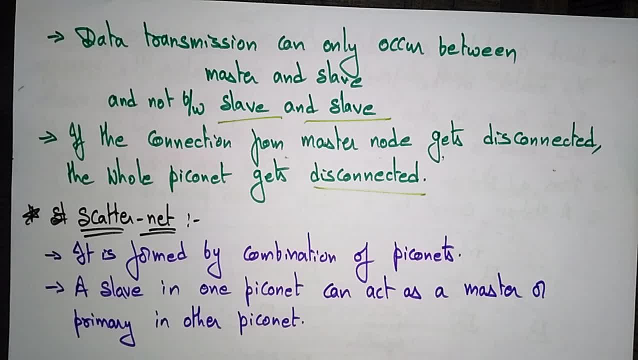 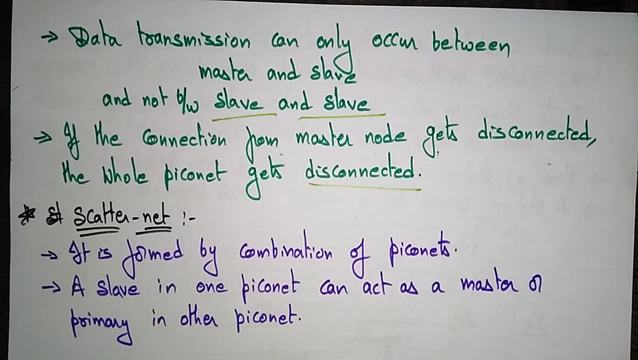 my lecturer. whenever the suddenly the power of something is happened, the system is shut down. what it will be do whenever the master node is disconnected? obviously the connection you're also from master will be disconnected. coming to the scatter node net. what is the scatter net? so far you have seen the arrangement of the piconet. only one master is there, so 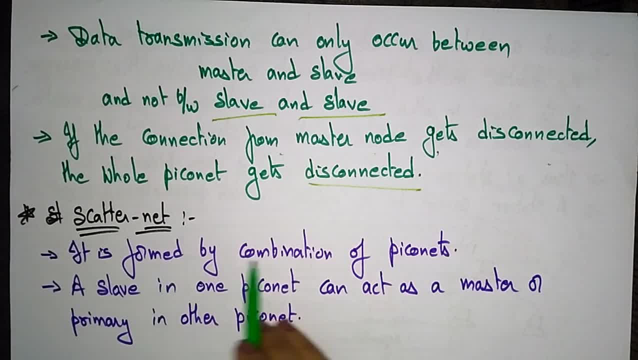 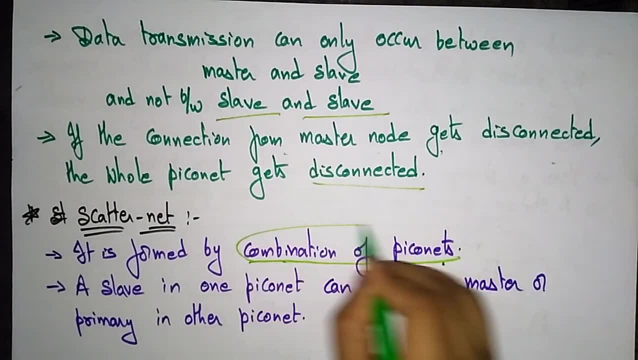 seven slaves are there. then scatter net: it is formed by the combination of a piconets. okay, we are seeing the scatter net is a combination of piconets. A slave is one. piconet can acts as a master or a primary to the other. 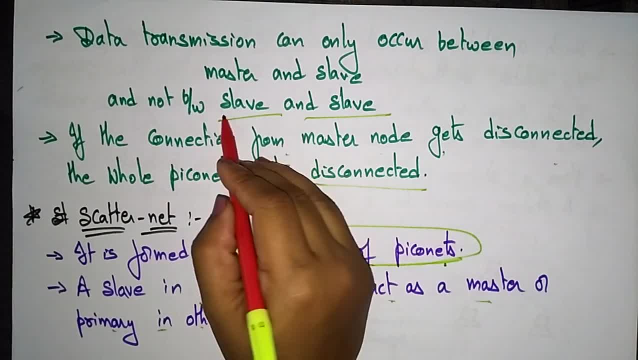 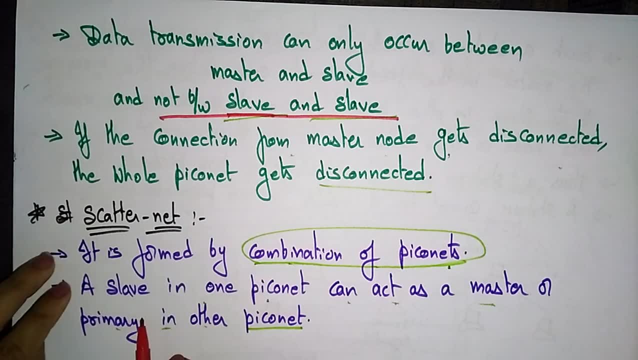 piconet. So did you observe here what I said? there should not be a connection between slave. data transmission should not be established between slave and a slave. But here, in this scatter net, what they are saying: suppose a slave in one piconet, So in one piconet, this is acting. 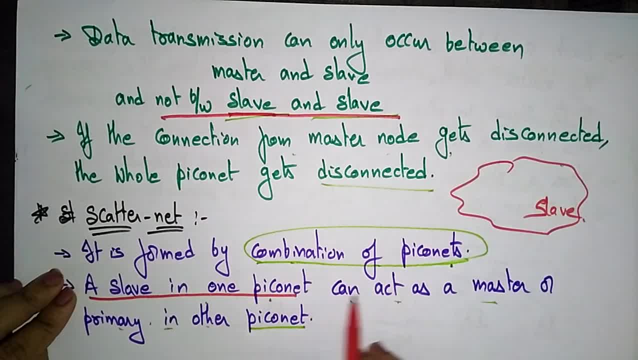 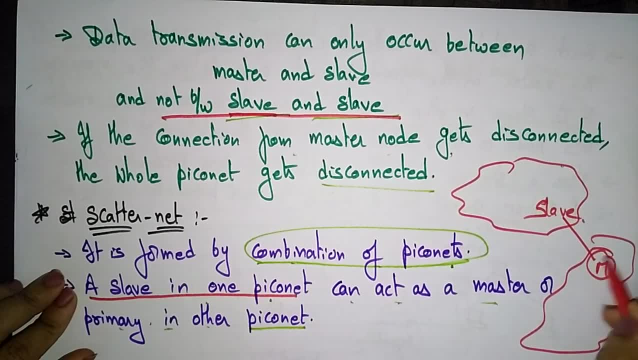 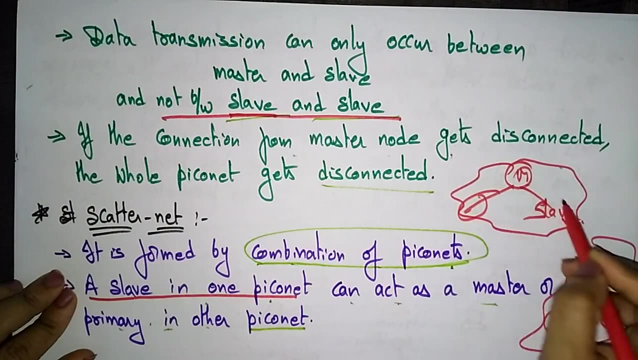 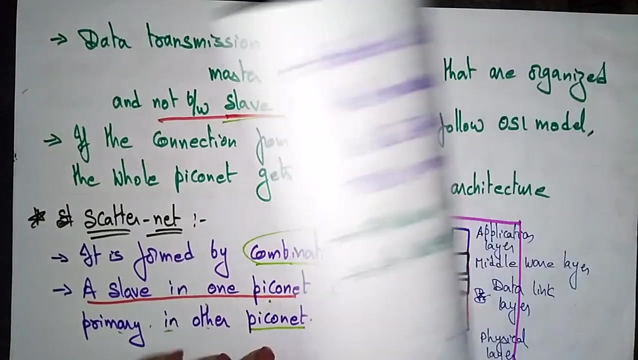 as a slave, can act as a master. So it can be act as a master in another network. The slave in one network can act as a master in the another network. This complete structure, you call it as a scatter net. Such a station or a node can receive message from. 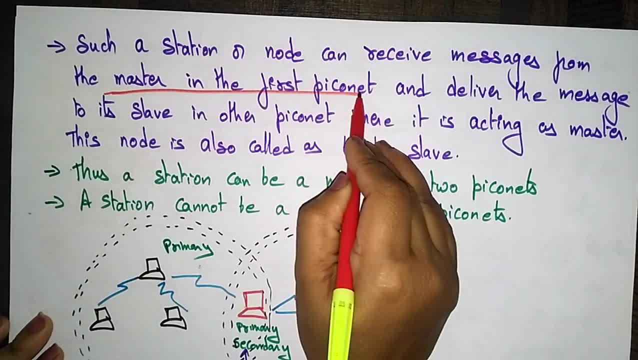 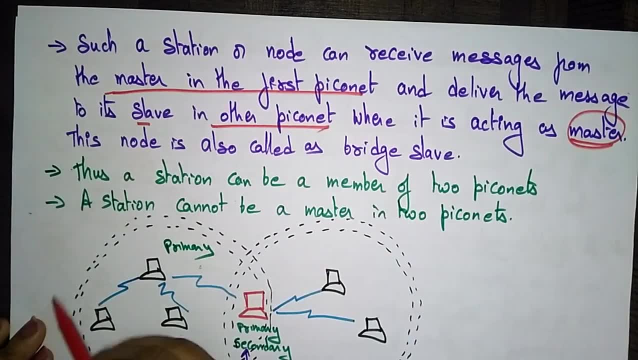 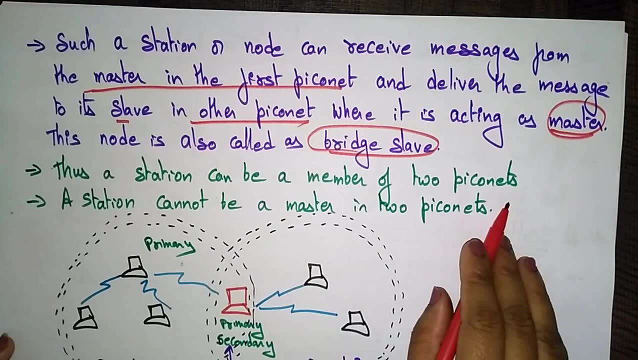 the master in the first picconet, from the master in the first picconet, and deliver the messages to its slave in other picconet where it is acting as a master. This node is called as a bridge slave. We call it as a bridge slave. Thus a station can be a member of two picconets. So a station can be. 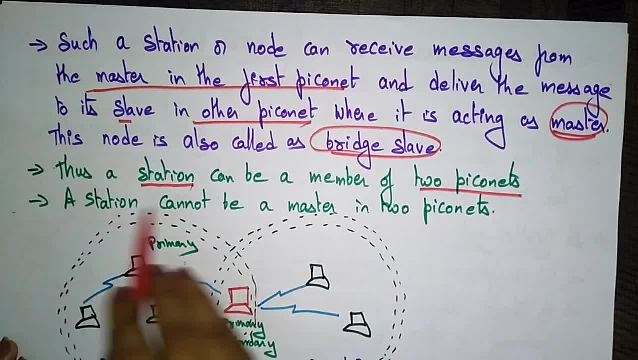 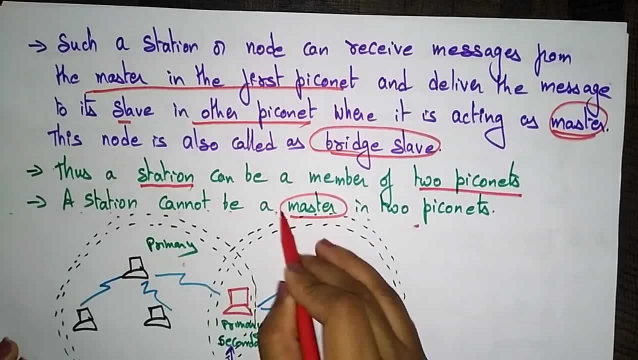 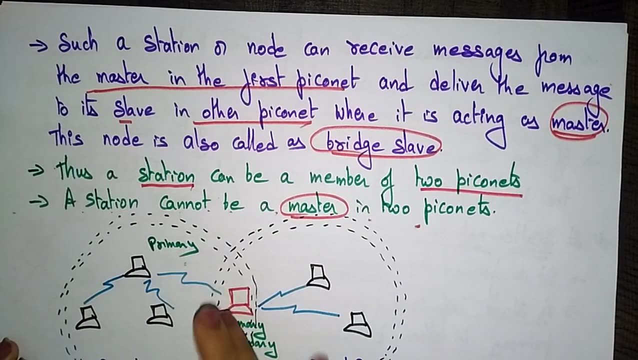 a member acting as a member of two picconets. A station cannot be a master in two picconets. but one thing you have to remember: that the station cannot be a master in two picconets. It can't act as a master in two picconets. In one picconet it can act as a master, but in another picconet it. 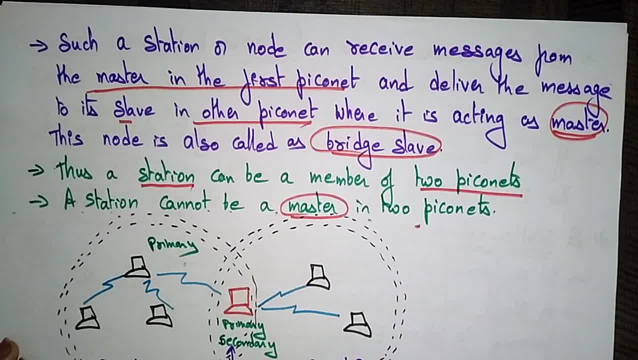 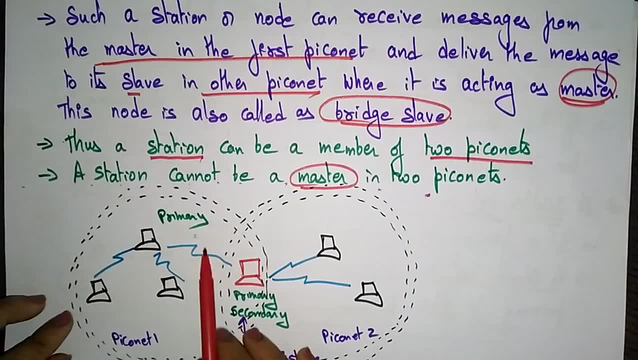 can't act as a master. Only in one picconet it can act as a master, because in another picconet it is a slave. So see the structure of scatter scatter net. So this is one picconet 1 and this: 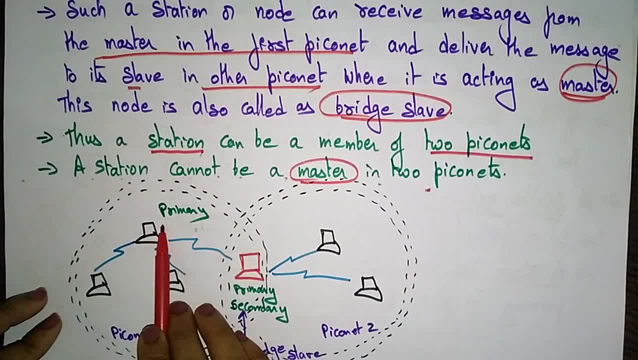 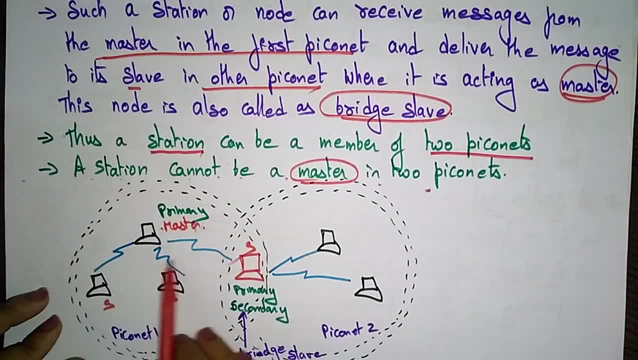 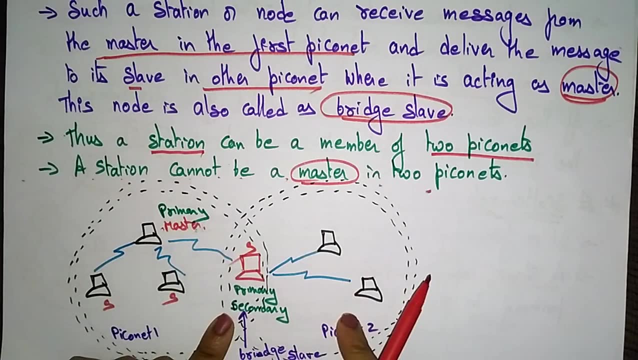 is another picconet 2.. So here this is a primary, that is a master. The master is sending the information to the slaves. So in another picconet, this slave which is acting as a slave in another picconet, So in this picconet it becomes the master. 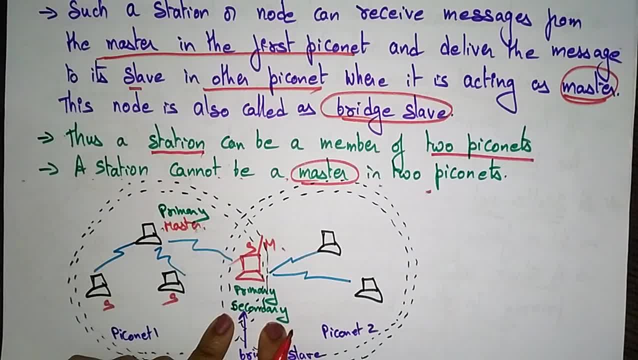 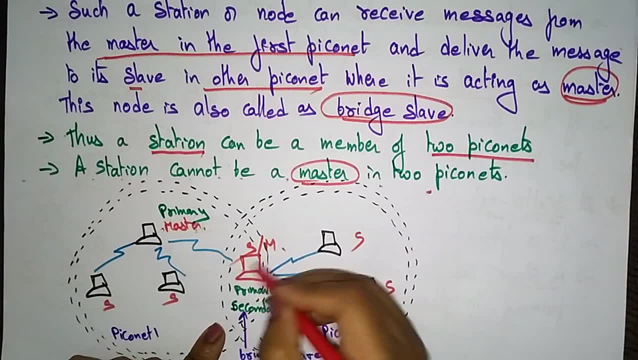 which is a primary or secondary, and it is sending the information to all the slaves, communicating with the slaves. So this system, you call it as a bridge slave. So this bridge slave is a bridge slave. So this bridge slave is a bridge slave. So this bridge slave is a bridge. 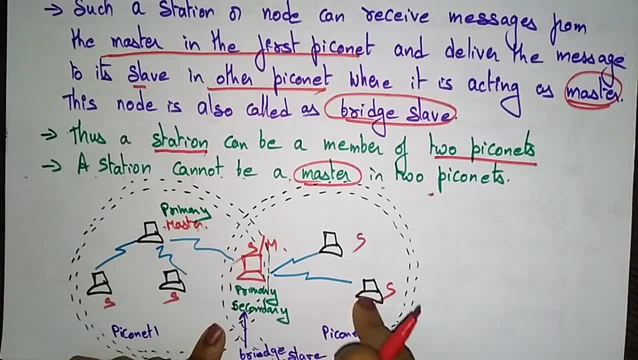 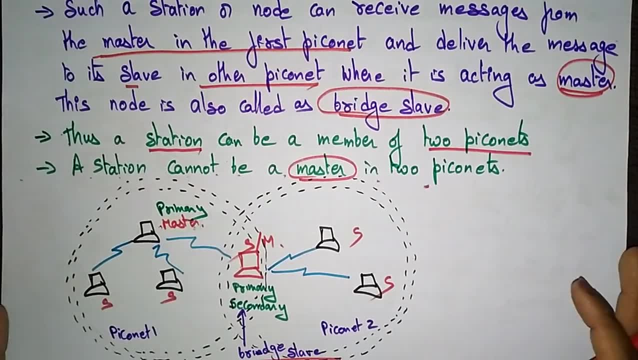 slave. So this bridge slave cannot be a master in two picconets. In only one picconet it is acting as a master, In another it is acting as a slave. So this type of communication arrangement- you call it as a scatter net, So the Bluetooth technology can be arranged in the form of picconet. on the scatter net. Thank you,